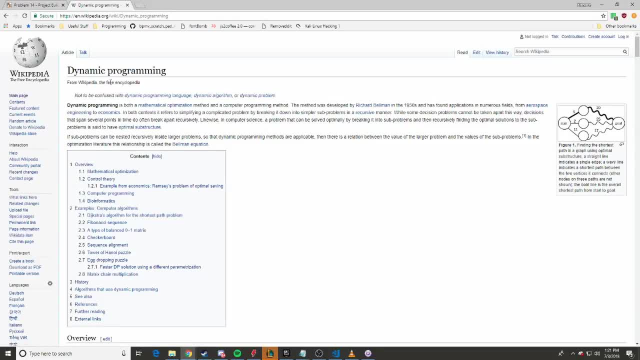 And the TLDR is dynamic programming. So basically taking a problem and breaking it down into subsections, Usually in a recursive manner, as it says here, And the memoization part is, what we're going to be doing is we're going to be taking the result that we're already calculating and we're going to be storing that result, So if we come across it again, it'll be very efficient. However, this is at the expense of memory. 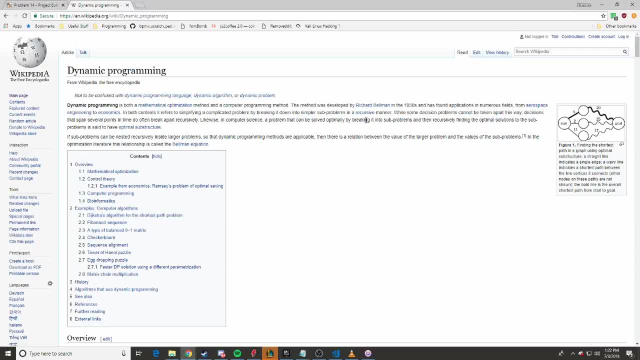 Although we do get to save a lot of time, And I'll show you how fast we get to save, How much time we get to save Roughly. However, I'll also show you how much memory, And so let's just go ahead and get into the code. 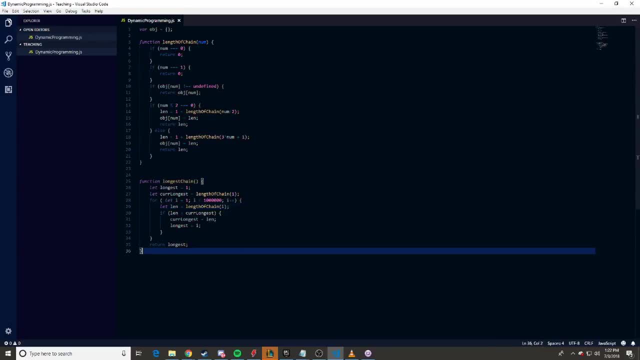 So, as you can see, here I have a predefined thing, And this is what we're going to be building, So I'm just going to start from scratch. So that is what our end result will look like. Feel free to pause the video now and go ahead and see if you can figure out what it does on your own. 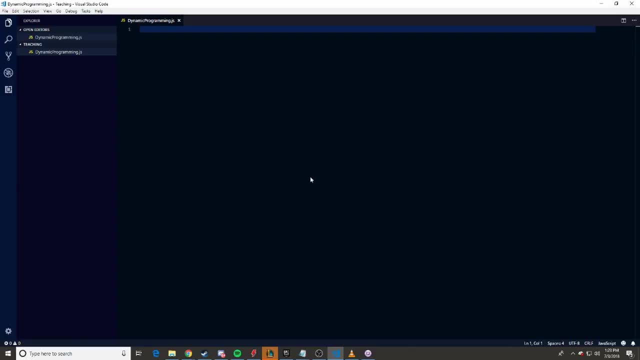 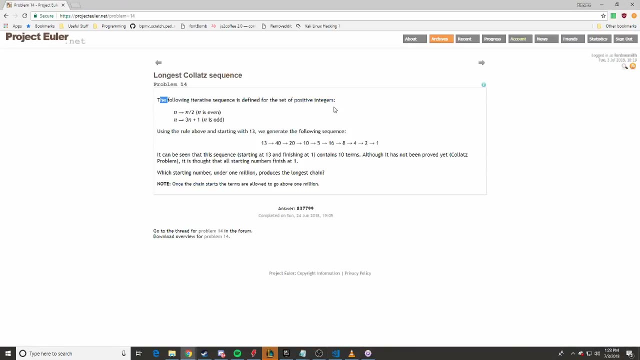 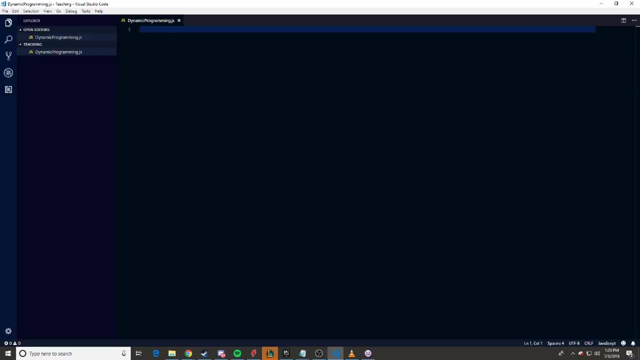 And why it's that way. And so, first things first, I'm just going to show you a quick example of how to solve this project. Euler question Over here With the basic example, a way to do it, but it's not going to be a very efficient way. 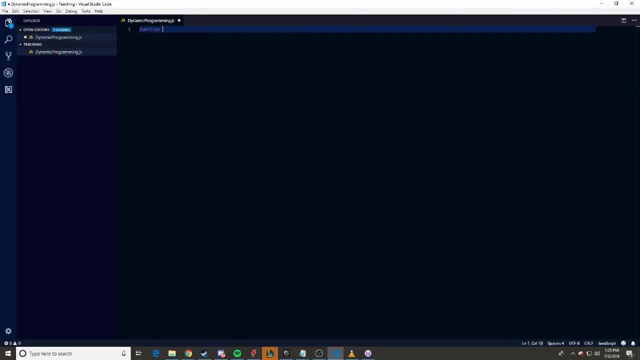 And I'll show you why in a second. So we're just going to create a function length of chain And before actually I get into this, I should note: So here's our goal. So the problem states the collapse conjecture, which, if you don't know what that is, 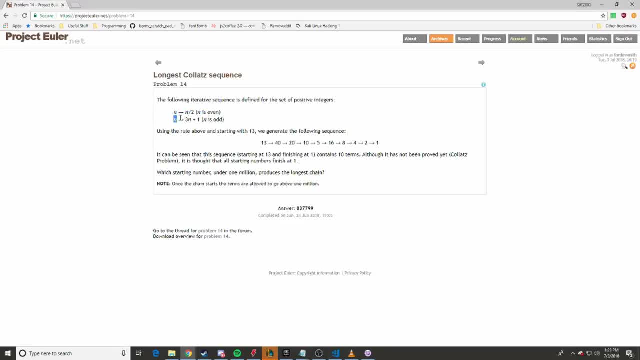 it's. you take a starting number, If it's even, divide it by 2.. If not, multiply it by 3 and start at 1.. And the collapse conjecture states that you will go through a sequence, And this can go up to hundreds of. 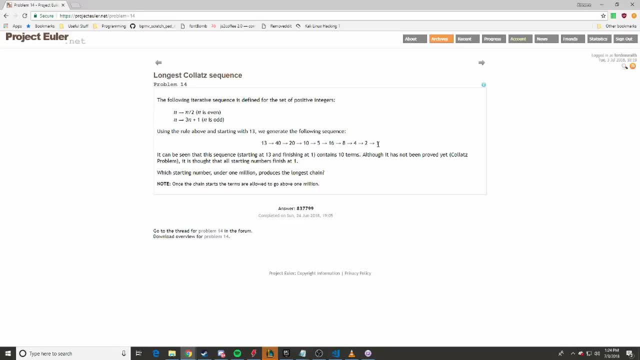 chains long And you will always end at 1.. And it actually has been proven that all numbers between 1 and a million end at 1. And due to just rigorous simulations already by people. So we're going to go ahead and have that assumption that they do. 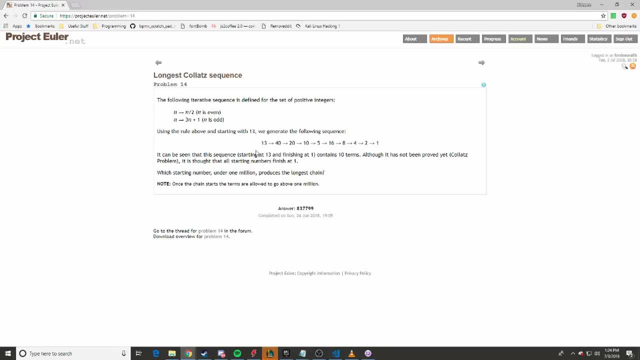 all end in 1. Because this is an unsolved problem and people have done much further than 1 million to thousands of digits long, Actually seeing whether or not it actually does follow, And anyways. so, as we can see, this goes through, say we start at 13,. this has 10 terms. 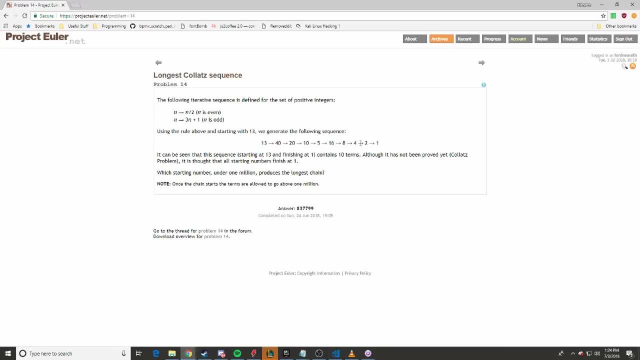 in this: 1,, 2,, 3,, 4,, 5,, 6,, 7,, 8,, 9,, 10.. However, it goes through 9 processes, So we can count either of these. What this problem is asking is what number produces. 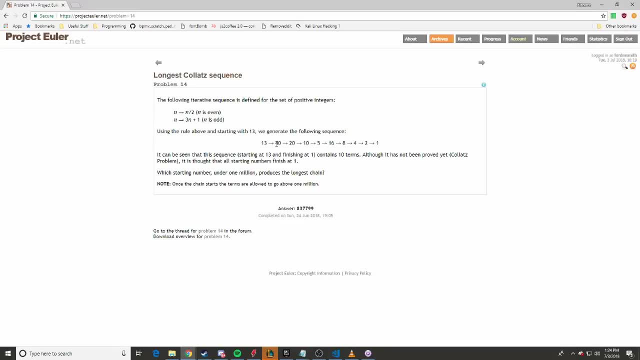 the longest chain, Not how long is the longest chain. So as long as we make sure we consistently count, either by incrementing like 13 to 40 as one step, or as each individual 1 counts as 1, we will get either 9 or 10.. 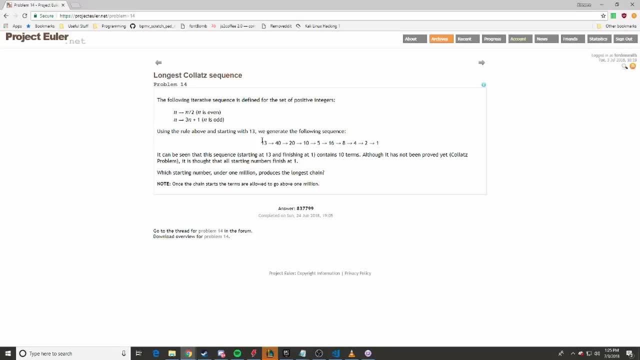 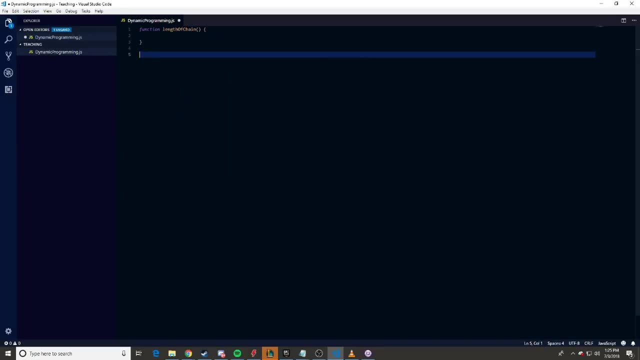 But since the way we're going to design it is, it will do it consistently. it won't make a difference in the end result. So that's the first thing that we can know. That's the first thing that we must know. Another thing is: is the best way I can think of doing? 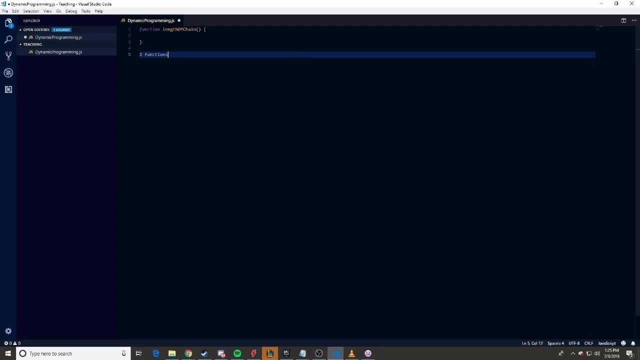 this is just creating two functions. The first will grab the length of chain at a number, And so, basically, that's what this is going to be: We're going to pass in a number and it will calculate the length of the chain. You know, fairly easy. 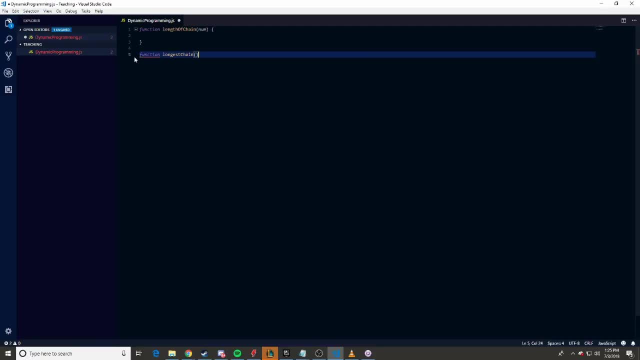 We're also going to create another function, Longest chain. This is just per phone preference. You don't have to put it into a function, but all the code will still be valid outside of the function, And the reason for this is this is just going to go iterate through. 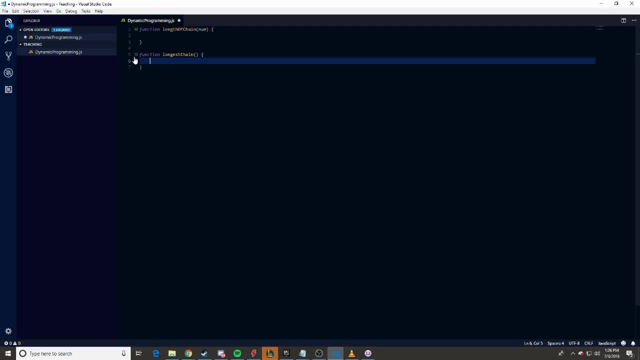 all the numbers and then pass it. I like doing this modular kind of thing. I mean you could technically put it all in one, but I think it's just a lot easier to think about it and edit it when it's you know. 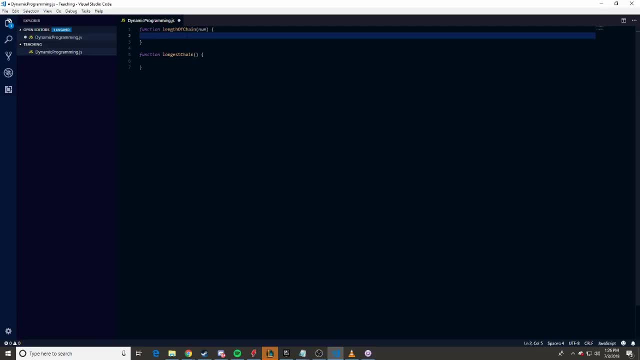 nice like this. This also follows the dry CS tips. You know, don't repeat yourself. So, anyways, we're just going to go ahead and do this. Like I said, this is, you know, kind of expecting that you already kind of know some basic. 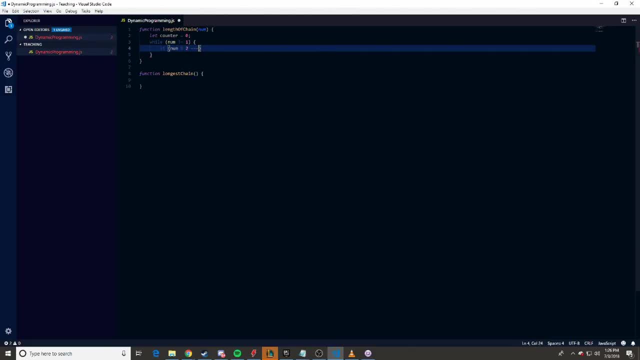 programming design. So I'm not really going to go into too much detail of what's going on here. However, I will do a brief explanation When I finish it. Also, this is a kind of different kind of thing that I'm doing, And so if you guys have any tips or you, 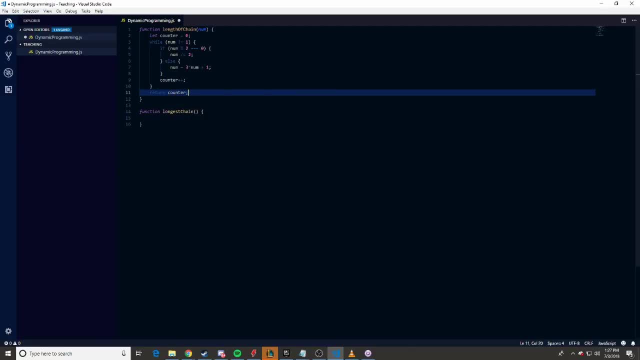 didn't like something about it, you just go ahead and let me know in the description and we'll see how we can improve it from here. You know I'm still kind of new at this stuff and I want to know how I can get better, and constructive criticism is always appreciated. 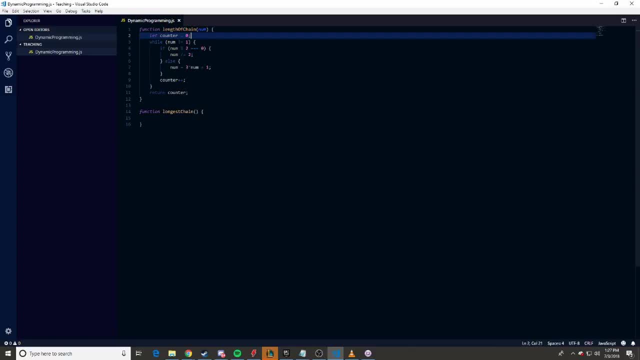 Anyways. so what this function is doing is, this is a counter, and this counter is going to keep track of how long the chain is, the current chain is, And the reason we're going to be using a while loop over a for loop is because the while loop will keep doing it until we hit this condition. 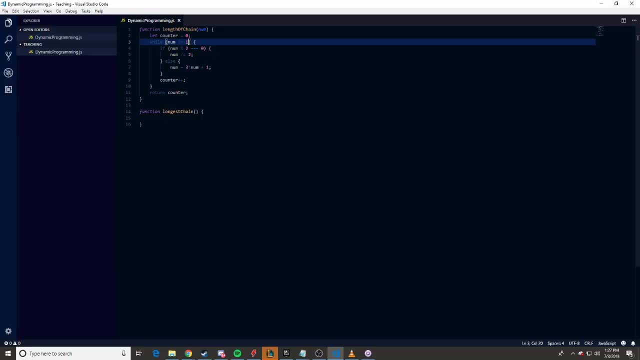 While the for loop. you know it's typically, I mean, you can do the same thing with the for loop. It's just easier to write with the while loop, Anyways, and it's like: if the number is divisible by two, divide the number by two, otherwise it's odd, and just do multiply it by three and add one, and then increase the chain, since it does not equal one. 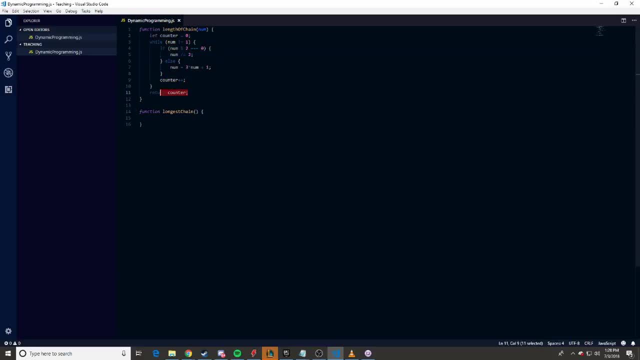 And then we're going to, and then, once this is all done- this will be the length of the chain and just return the length of the chain. Then what we're going to do is we're going to create: let longest equal One, let current longest. 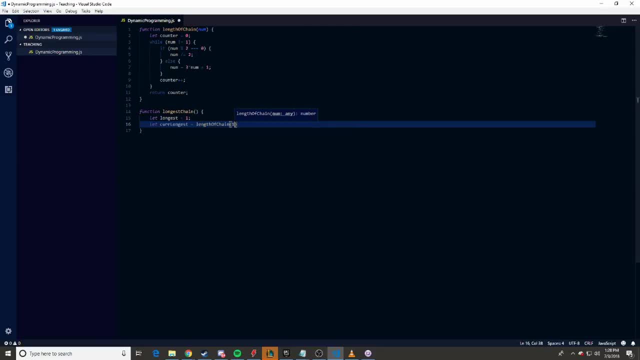 equal length of chain of one And four. let i equal. we want to start this at one, Yeah, And zero, zero, zero, zero, zero, zero, yep, And i plus plus. And the reason we want to start at zero, we don't want to start at at zero is because, say we pass in zero to here, it'll go on infinitely. 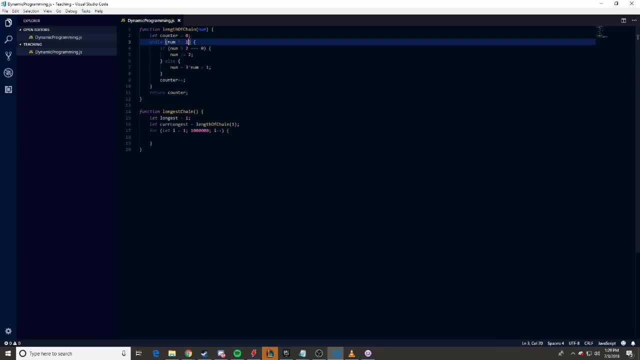 And the reason is is because, whether, no matter what, you're always going to be either dividing a zero by two or multiplying a number by zero. Um, Here, hold on. All right, Let me refresh that You're always going to be again. 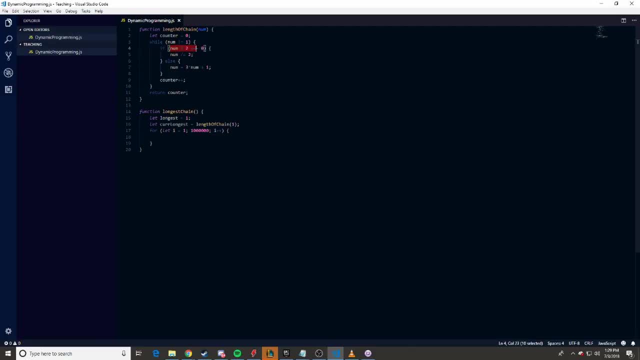 So, since zero, it's always going to be um divisible by two, which is what this is saying, um, because you know it's can have. this is just checking to make sure that there are. The remainder equals zero. 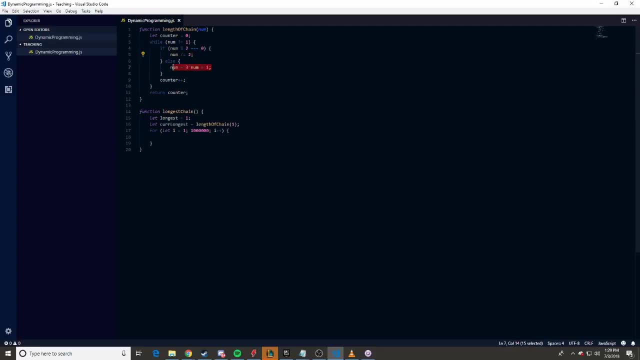 And if you do zero divided by two equal zero with no remainder. so it's always going to be running this statement here, So it will never reach this statement, And then also it will be continuously just doing this loop over and over and over and over again. 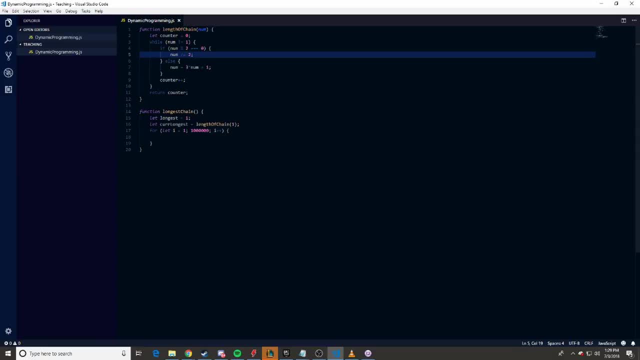 Because it will never equal one ever is. 0 divided by 2 is just equal to 0. So that's why this will create an infinite loop and why we want to start it at 1 and not 0.. Anyways, then, we're just going to do the basic. 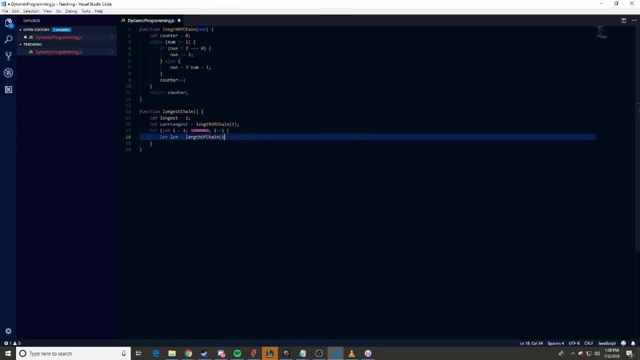 you know, grab the length of the chain at i, then if I cannot type today, length is greater than currentLongest. then currentLongest equals length. and the reason I didn't just do, like you know, put this here and there instead, is because that you know, if we store it once, you know we don't have to. 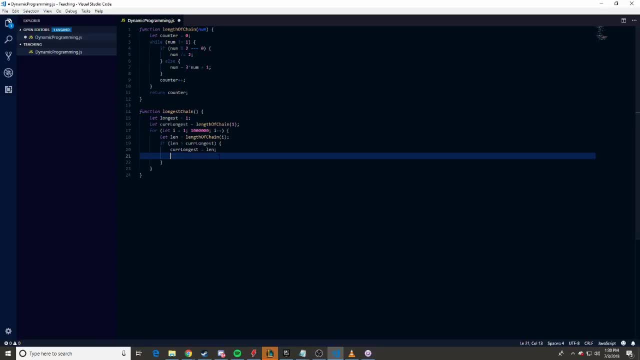 do the computation twice over, Which, if we did, we'll make this even longer than it already will be, and I will show you. And then we're going to set longest equal to i, And at the end of this, all we just want to return. 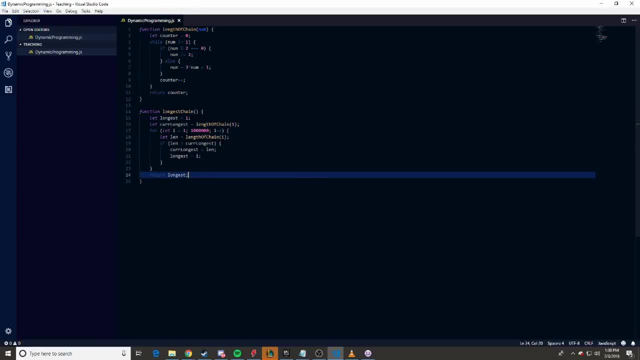 the starting index. So, basically, this is going to store the starting index and this is going to store the length of this. This is not going to be the starting index. I mean 1 is the starting index and the reason we set it as 1 is so we have a default value. 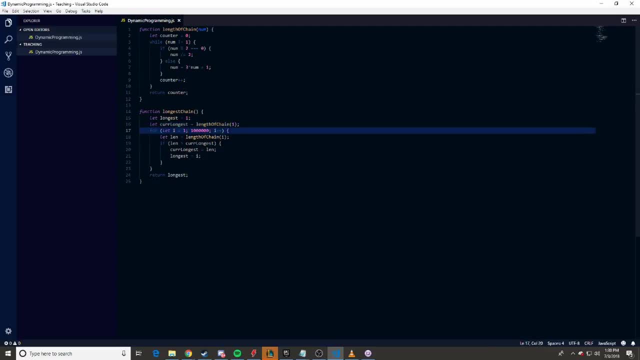 that it can compare to. that's part of this. Otherwise, say we set the longest to something that's outside of the scope of this range and that number, just coincidentally, is the longest chain, Then you know it'll always fail and it'll just return that. Or say you know you have a function. 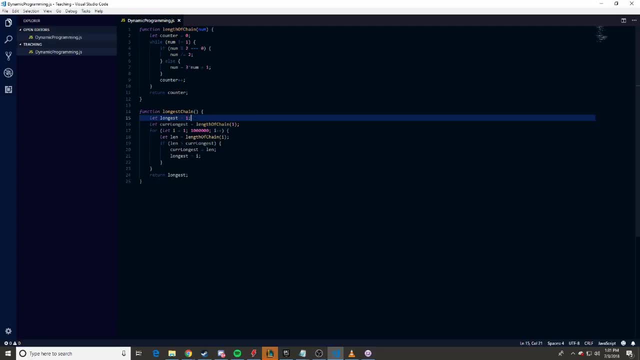 where you're trying to figure out what's the biggest value in an array and you set the default to 0, what's going to happen is, if all those numbers in the array are negatives, 0 is going to be the highest one, So even 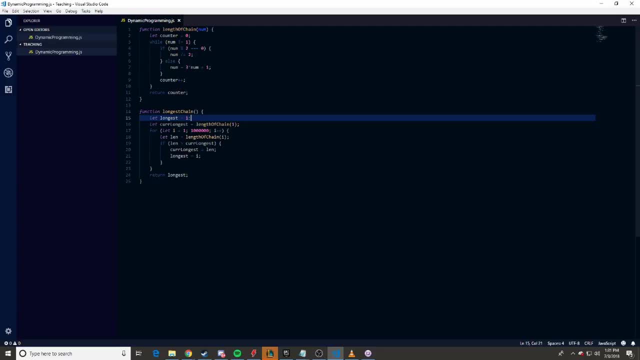 though 0 is not part of that array, it's still going to return 0. And that's why you always want to start it with one of the indexes, or you start with the lowest possible integer value or the highest possible integer value. You know, and it depends on what you're trying. 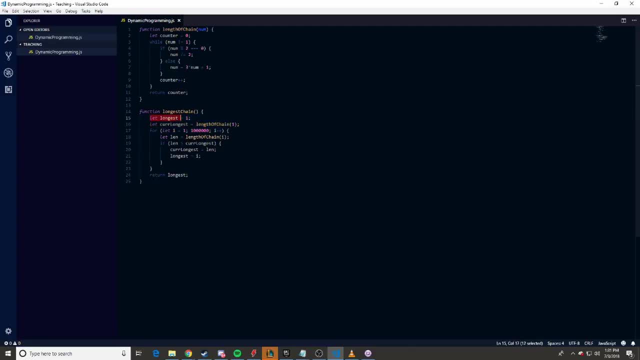 to do Anyways, but this will store the starting number you know, like 13,, for instance. Say that's the longest one you know. it'll store 13 there, and then the length of 13,, which would be 9 or 10. And then what it'll. 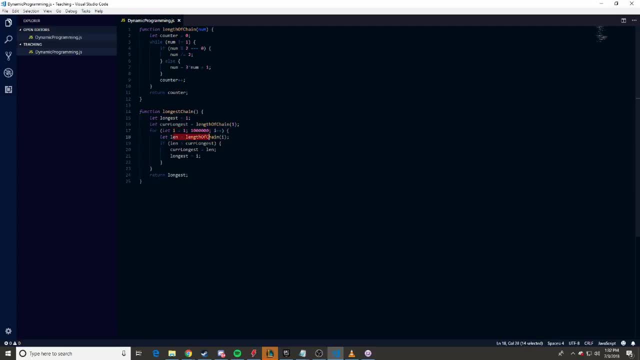 do is it just iterates through every number and grabs the length of the chain at that number and if the length of that chain is greater than the current length of that chain, just store it and then return whichever one's the longest You know. pretty simple. 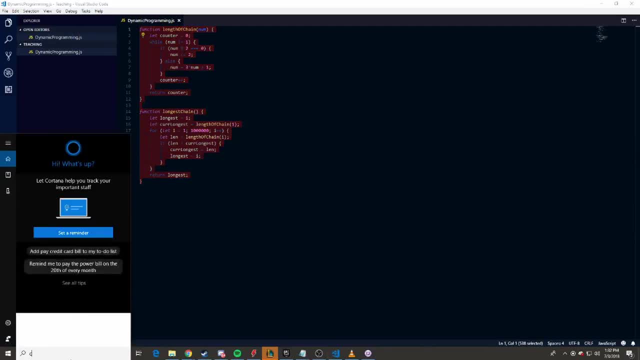 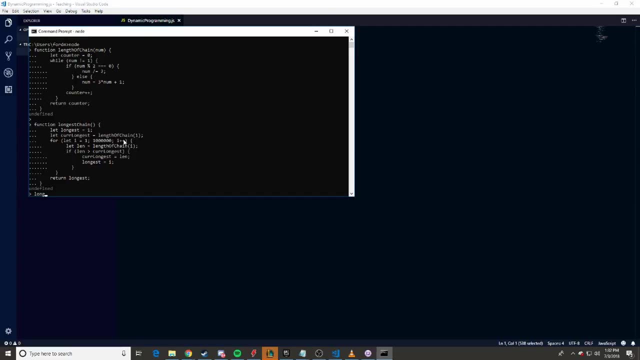 However, if we run this in the command prompt and then we do longest chain, as you can see, it's going to take a while. I don't have this kind of patience. So what are we going to do about it? Well, we're going to use, we're going to implement dynamic programming and memoization. 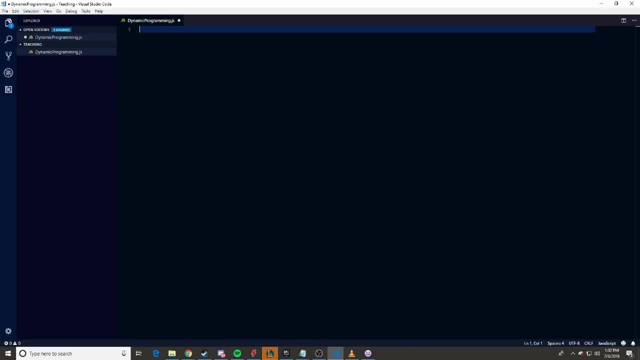 Like I said earlier, dynamic programming is you split up an issue into smaller subsections, And we're going to do this with recursion- And you'll see why we'll do it with recursion in a minute- And then, on top of that, we're going to implement memoization, which is basically 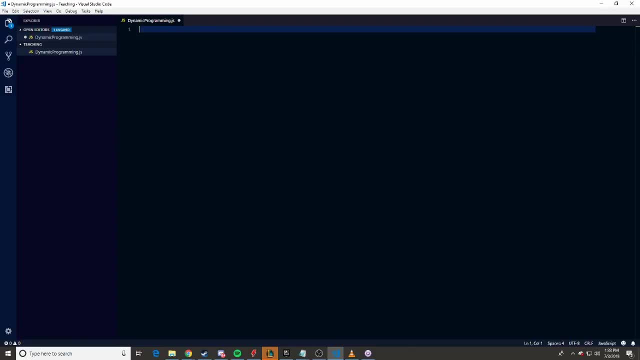 where we're trading memory for speed. So with dynamic programming we're going to compute, you know the length of the chain And if we come across that, say 27,. you know, not necessarily, but say that goes to somewhere down the line, to 13. Okay, instead of doing, 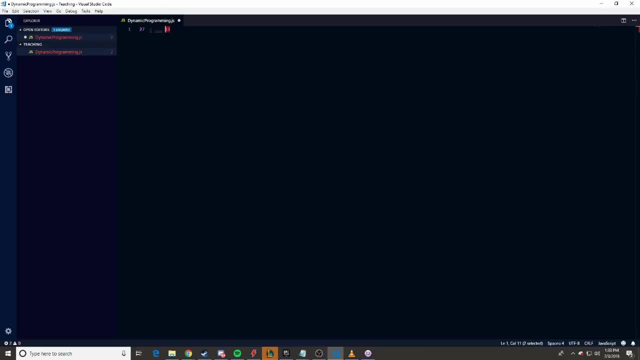 the computation for 13,. over and over and over again. we can store 13 and just add it to this previous thing. So we're saving the rest of this chain computing. that And all, Although it doesn't seem very big when these chains get hundreds of chains long like hundreds. 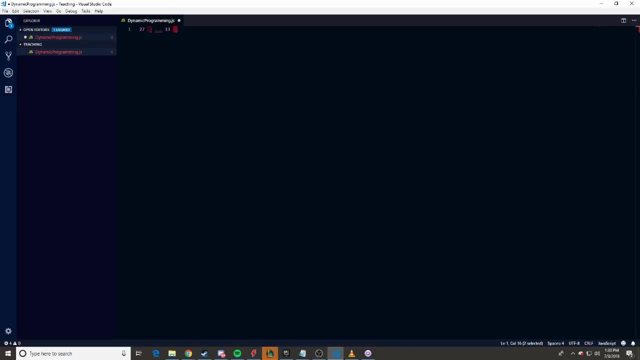 of whatever long, that can become very computationally expensive, like we just witnessed where it didn't finish. So if we just use up a bit of memory and store this value, we can add it together. So now, whenever something comes to 27,, we can forego having to do all of this again. 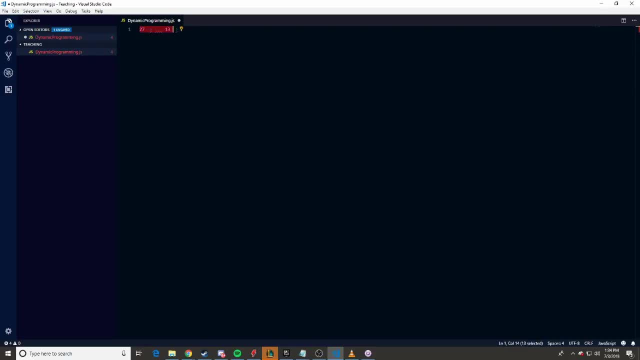 And if something whatever led to 27,, we come across that again, all of that is saved, which, you will see, is vastly faster. So we're going to do, or actually only, and the good part is, we don't even need to touch. 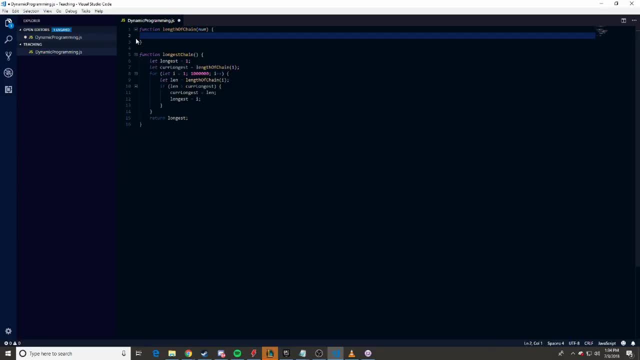 longs chain. We only need to change length of chain, which is where all the computation is occurring. So, first off, just as a safety measure, if we pass a number that's equal to zero, we're going to return zero, Just as a flat case. make sure nothing goes wrong. 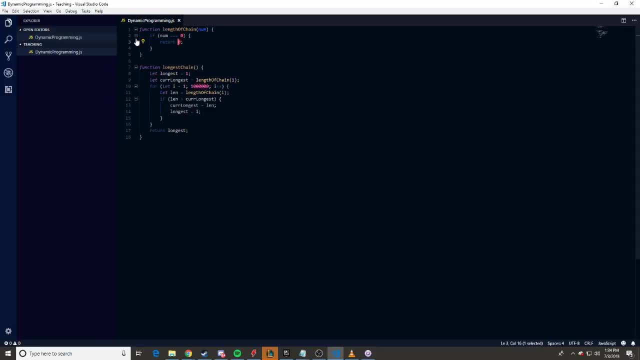 If we wanted to, it would probably be better to set it to the lowest possible integer value, just so everything is higher than it. technically speaking, almost everything. However, in the scope of this, it's not really going to matter too much. 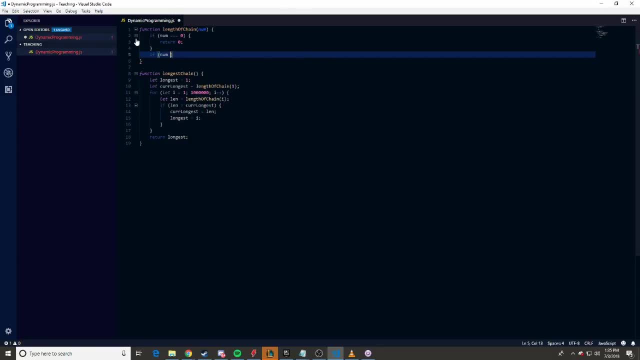 However, in some projects it might- And then in recursion we're going to have our base case And then we're going to have our base case And self-explanatory. when you're doing recursion, you always, always have to have. 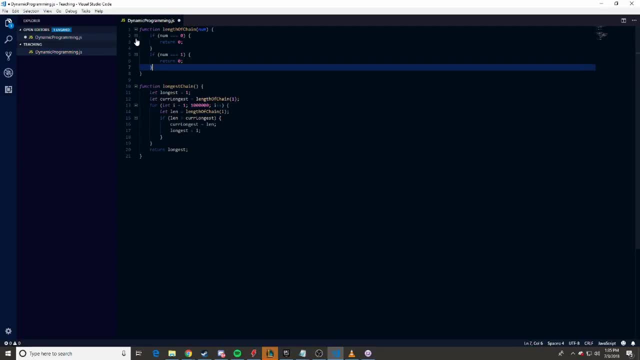 a base case. Otherwise, it will be infinite and it will never end. However, this is where we're going to start implementing memoization, And what we're going to need to do is we're going to need to create an object that will 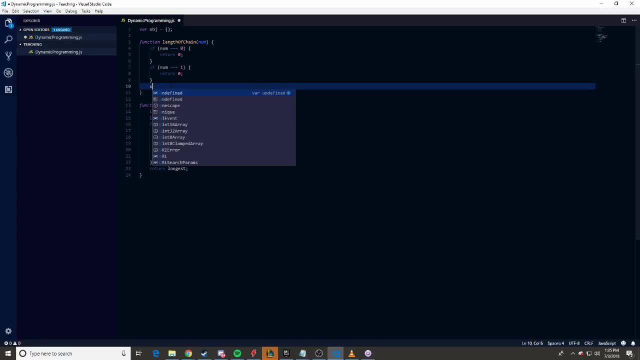 store all the information and it will be easy. So if the number that we come across Ugh Is equal to zero, It's going to be zero. It's going to be zero. It's going to be zero If it's in the object, which means that it is defined. so this is saying: if we have come, 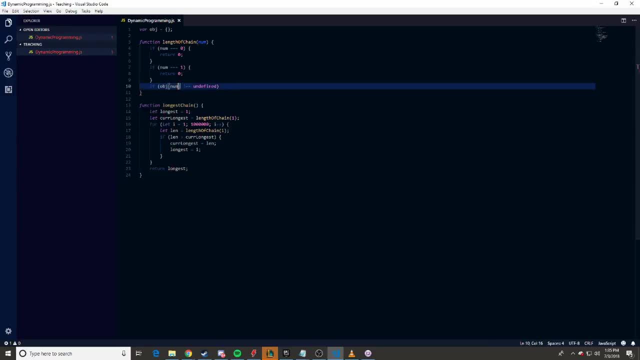 across this number before because it will be defined. then we're just going to return that number And then we go on, just break it a little with collapse conjecture style. If Yes, It's divisible by 2.. oops, then the length is equal to 1 plus the length of chain num divided by 2 and 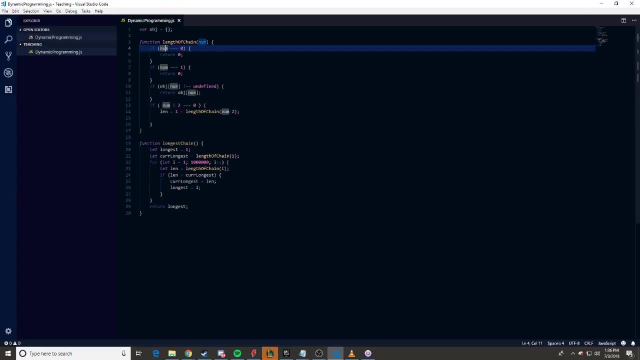 so if you're not familiar with recursion, I suggest you go check out some tutorials. or if I this, but later I will- I should relatively soon have a tutorial on recursion out there and I'll show you like when it's good for and stuff, and so you know it's just easy. you know we're just continue on and we're going. 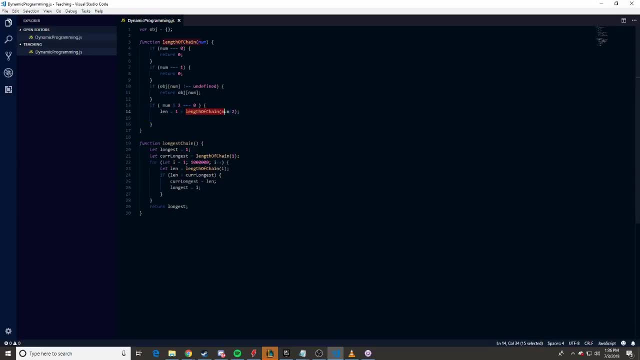 to add 1 to the length of chain. so basically, this is where the dynamic programming part comes in. you know we're going to compute each thing in a subsection, so so if it passes the this part of the collides conjecture, we're going to pass it again, and then we'll do this over and over again until we reach. 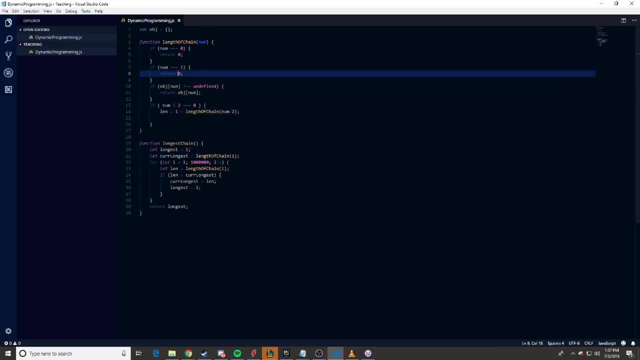 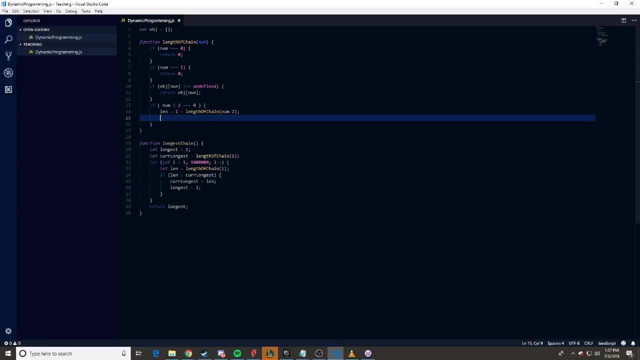 do this. this will save a lot of that computation time. so that's my cat. I don't know if you heard them, and then we're just return its length. so it continuously do this over and over and over again until you know everything's, it's. 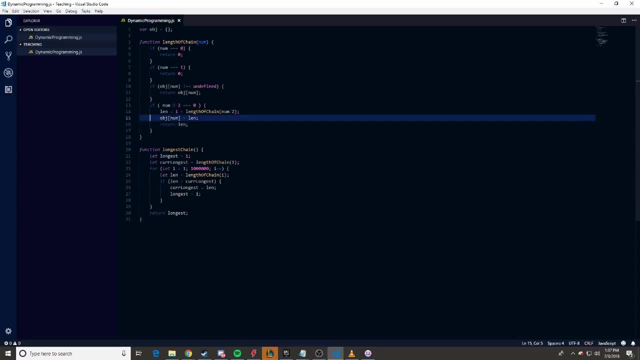 either you know reaches one, and then it's done. that's the length of the chain, or it comes across something it's already been to and it'll return that instead, And then it's the same thing if it's not divisible by two and length is equal to this except. 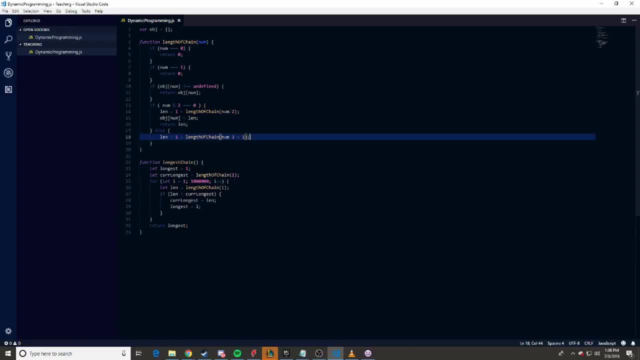 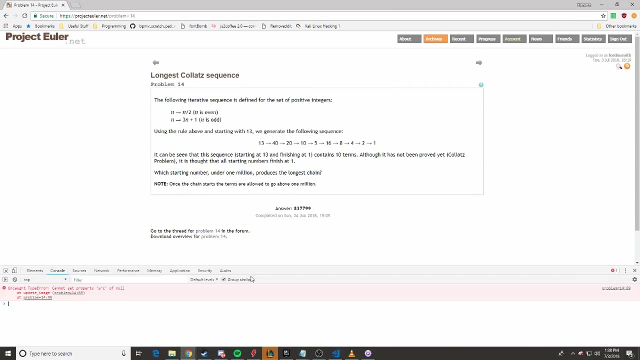 it is num times three plus one, And then we're going to do the same thing. just object of num equals length, and then we want to return length, And that's it In fact. it's efficient enough that I will run it in my console without worrying about. 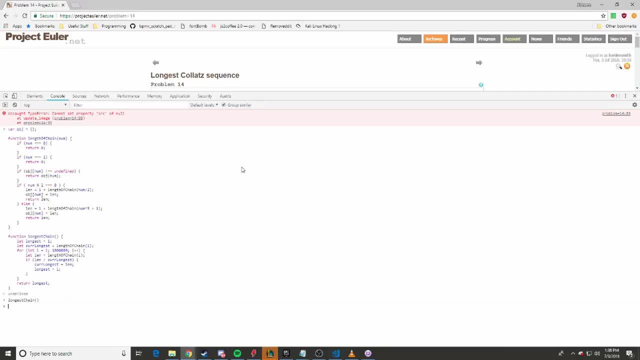 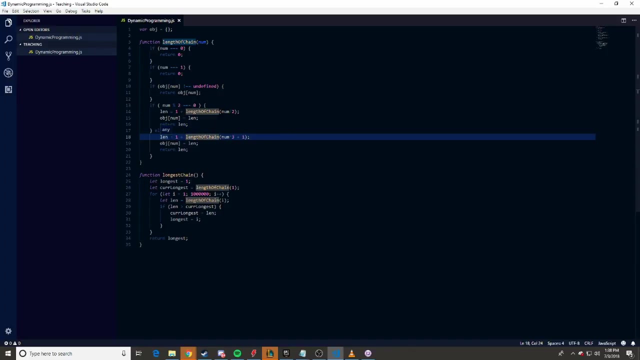 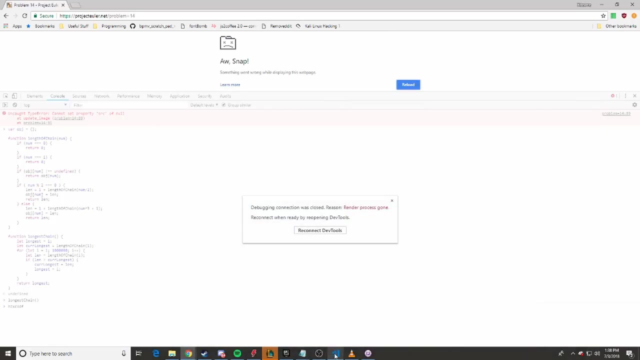 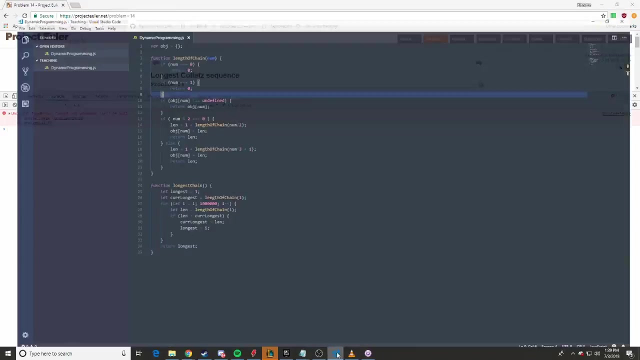 it, crashing it, And we'll do longest chain. and did I do something wrong? I did something wrong. Let's see here Where did I go wrong? Where did I go wrong? Just fine. Object of num equals length. return length. 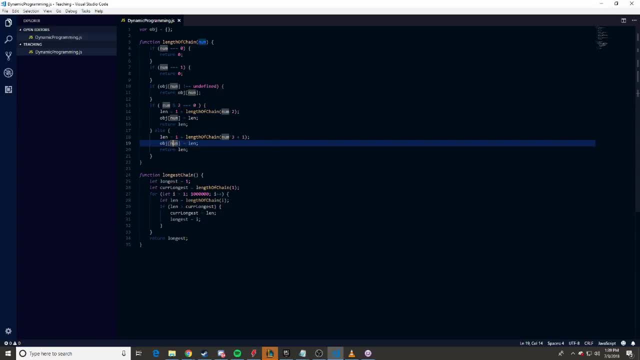 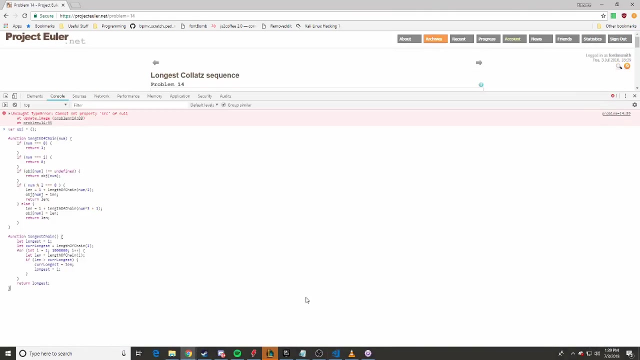 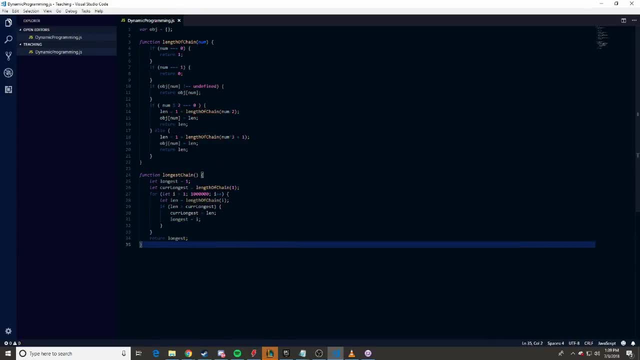